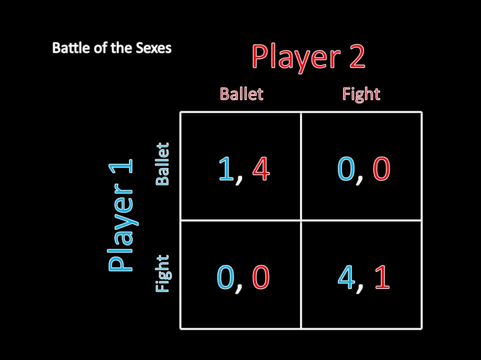 change the probability distributions that actually form the mixed strategy, Nash equilibrium. So if I gave you the solution to this game, you couldn't just tell me that the peer strategy, or rather the mixed strategy, Nash equilibrium, is to go to your more preferred form of entertainment with. 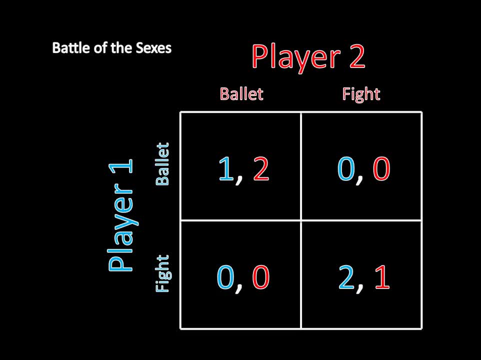 probability two-thirds, and go to your lesser preferred form of entertainment with probability one-third. That's not going to carry over to this situation. Likewise, I can make another minor change to this game: Move the ones to threes, And that's not going to change the peer strategy Nash equilibrium, but it will change the calculation for the mixed strategy Nash equilibrium. 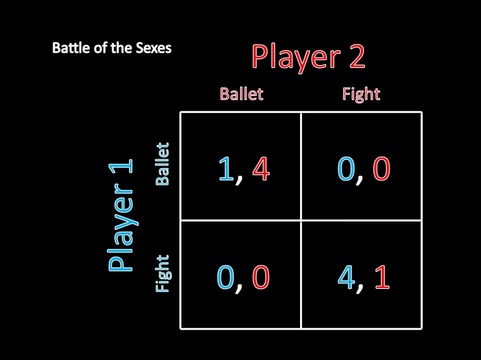 So, even if you'd solved the second game, that doesn't get you anywhere. when you try to solve the third game- And again I can make another slight modification, this time changing the zeros to ones, and you're in the same situation as you were before, Even if you've solved the first three versions of this game. 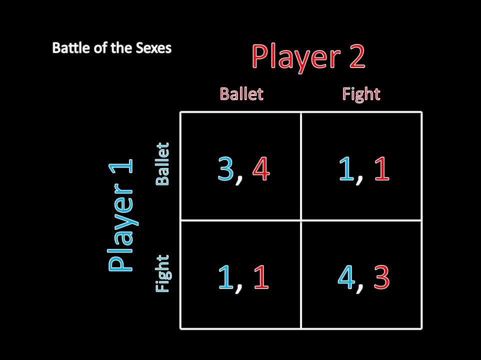 you still have to solve that mixed strategy Nash equilibrium again in this fourth game, And so that can be really frustrating if I'm giving you a lot of different versions of Battle of the Sexes and you keep having to redo the math on the mixed strategy algorithm every single time. 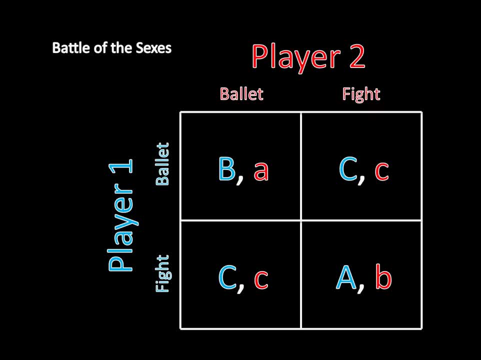 So it would be really neat and really convenient if, instead of solving games with numbers, we could solve them with variables like this, where we're representing A as the most preferred outcome, B is the second most preferred outcome and C is the least preferred outcome. 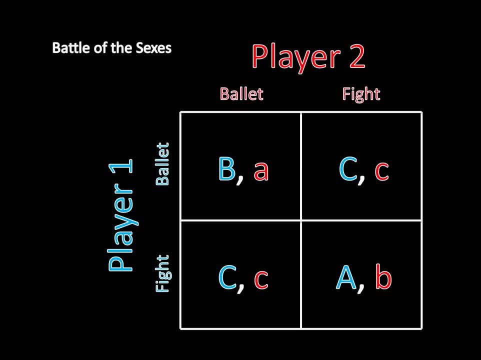 And if we could solve the games in this generalized form, then we could then specifically plug in the numbers for, say, this fourth example and turn these A's into 4's, the B's into 3's and the C's into 1's. 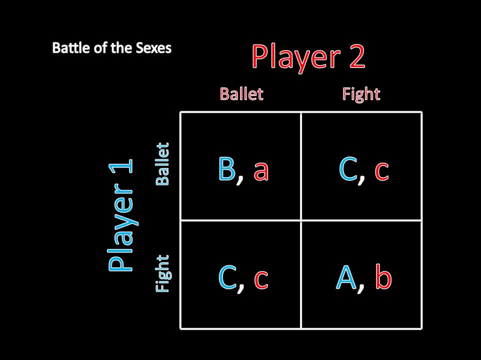 and then solve for the mixed strategy- Nash equilibrium- by just plugging those letters into a fixed formula that we've already come up with. So that's our ultimate goal and that's something that we're going to start looking at in the next video. 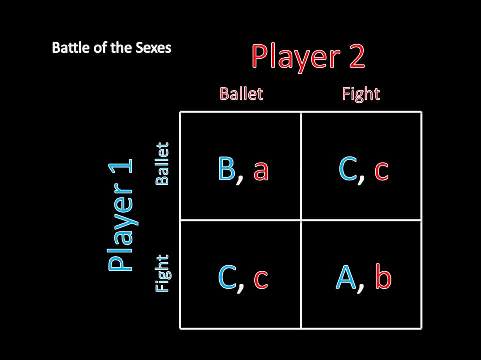 And after that we'll expand to looking at how the games change as the values of these parameters change, which is going to be a really interesting thing, and that's something that we'll be looking forward to even later in this this unit, But for now, it's important to actually have a firmer grasp of what a probability distribution is. 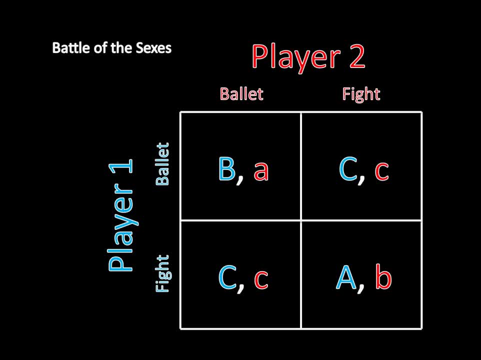 because we've been dealing with them implicitly all along, when we've been looking at mixed strategy, Nash equilibria- and it's important to actually understand what's going to be going on with those. when we switch over to the more complicated world where we're looking at letters in the form of variables instead of specific numbers. 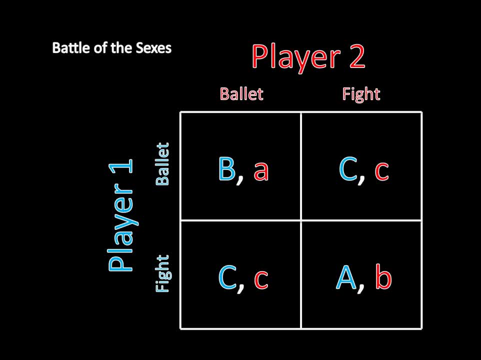 So a strategy, when we're talking about what we're actually going to be playing in the game, is a probability distribution. Sometimes it's a trivial probability distribution. So if player one is playing ballet as a pure strategy, that's still a probability distribution. 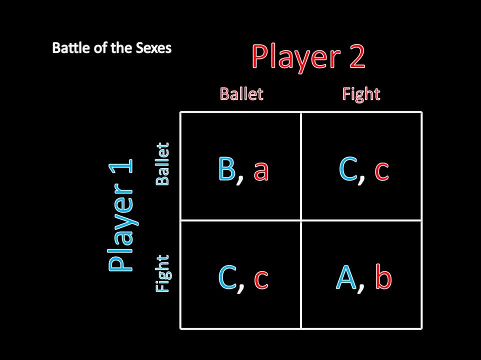 His probability distribution in the form of a strategy is to play ballet with probability one, or in other words, play ballet 100% of the time and to play fight 0% of the time. So those are trivial examples of what a probability distribution looks like in the form of a strategy. 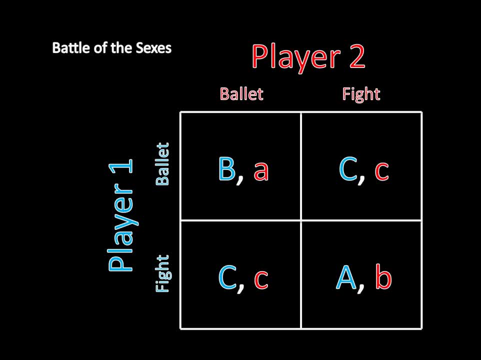 But then again we have the more intuitive and more interesting versions where we're actually mixing. where in the mixed strategy Nash equilibria of the original battle of the sexes game, I was going to choose to go to the fight with probability two thirds and the ballet with probability one third, when I was the man as player one in that original game. 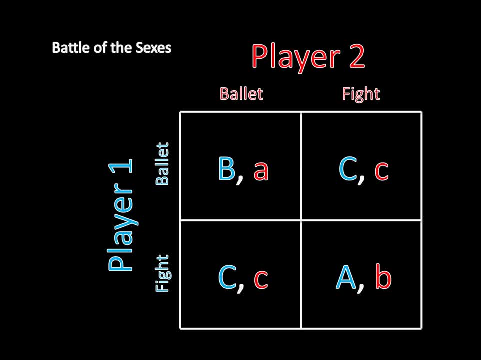 So we know that that sounds like a probability distribution, because I can choose to play something two thirds of the time. I can also choose to play something one third of the time, and that tells me exactly what I'm going to be doing every single time. 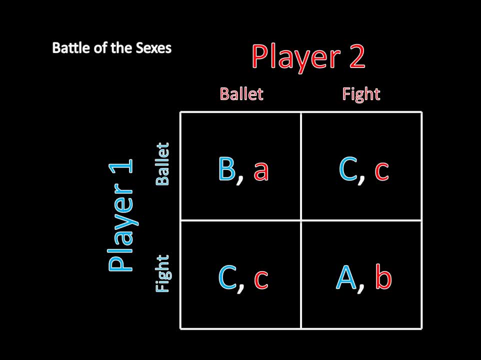 That's adding up to 100% of the time And that all makes sense. But what happens if, instead of giving you a probability that looks like one third, I instead gave you a probability that looked like b minus c divided by a plus b minus two c? 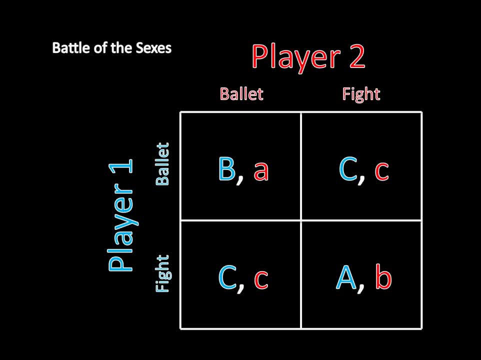 It's a lot more complicated and it's a lot less easy to just look at that and be like, oh yes, that's a valid probability distribution. So what we're going to have to do eventually is test whether things are valid probability distributions or not. 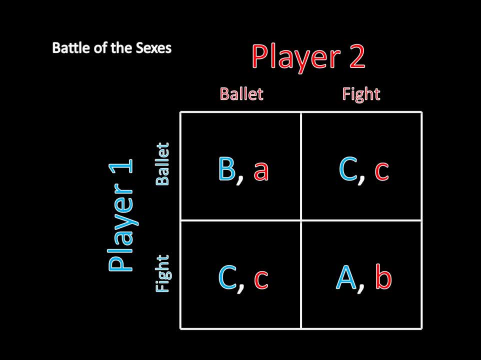 And what I mean by things there. I mean complicated expressions with letters instead of numbers, And so when we're going to be doing that, we need to actually have some sort of framework to go back to to understand whether something is a valid probability distribution or not. 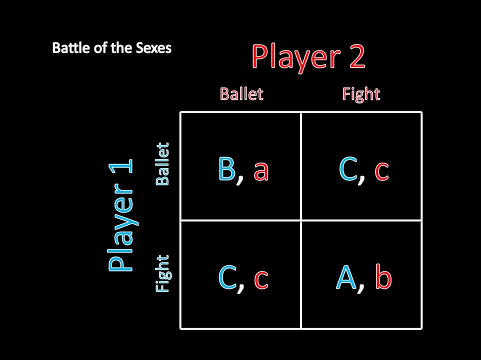 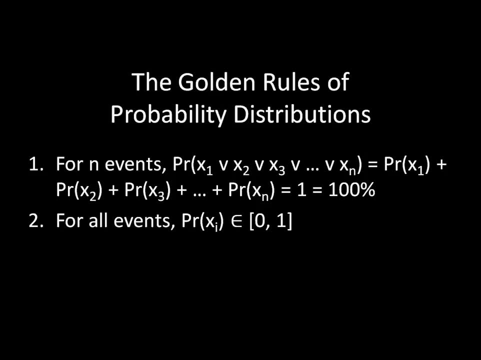 And so I'm going to now give you the golden rules of probability distribution. So there are just two things that you need to keep in mind whenever you're looking at a probability distribution, And I'll talk about some of the implications of these two rules in a moment. 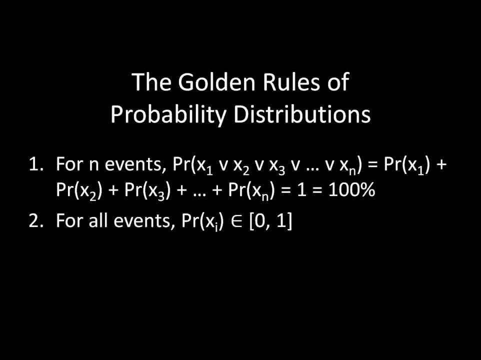 The first rule is that for n events, the probability of landing on any given one, So event one x1, or event two x2, or event x3 or and so forth, until you get to xn, The probability of those is the probability of x1 plus x2 plus x3, and so forth. 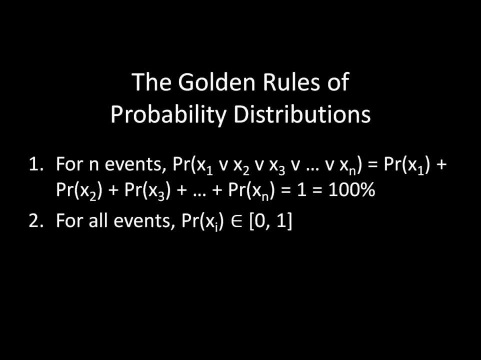 And those all have to sum up to one or 100 percent of the time. So what we're saying here is the events, in this particular case, when we're applying probability theory directly to game theory, when we're talking about events, we are referring to the probability that I actually play a particular strategy when I am mixing. 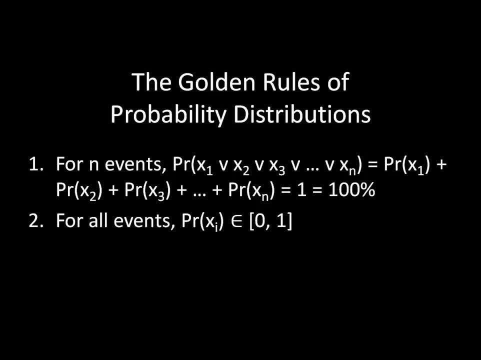 So an event may be play ballet, or it could be play football, And in this case, when we're only looking at a two strategy game, that's only the only two options that I have. I can only go to the ballet or I can only go to the fight. 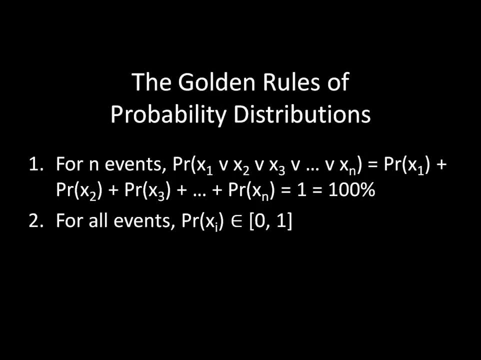 Those are the only two things that can actually result of my probability choice or my probabilistic choice when I'm randomizing in equilibrium, But you'll notice that two thirds and one third add up to 100 percent. So that's pretty good and that's pretty easy. 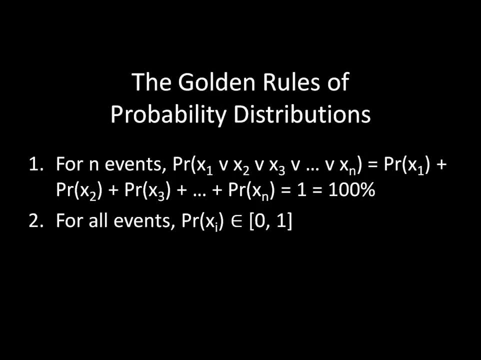 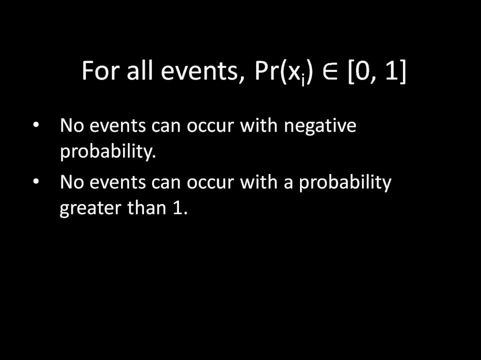 And then the second thing is that all events in my probability distribution must be between zero and one. So what that means? it means two things. It means that no event can occur with negative probability. I can't, for example, go to the fight 100 percent of the time and then go to the ballet negative 10 percent of the time. 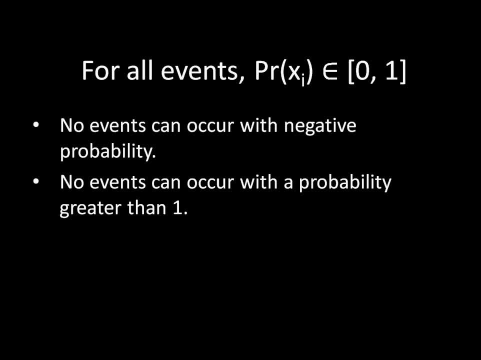 So that violates the rule that I'm choosing something with a negative probability when I said I was going to go to the ballet- negative 10 percent of the time. It also violates the idea that all of these probabilities have to add up to one, because 100 percent plus negative 10 percent adds up to 90 percent. 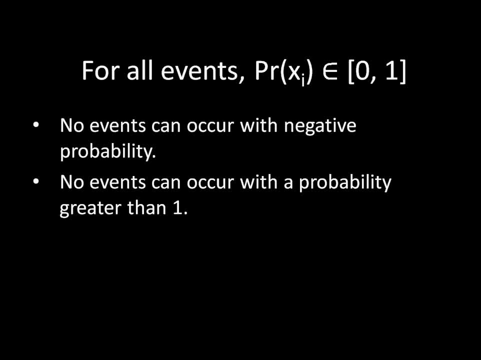 So that wouldn't work for that reason as well. But I also couldn't have a situation where I'm going to go to the fight. I'm in a situation where I'm going to the fight 100 percent, or rather 110 percent of the time, and I'm going to the ballet negative 10 percent of the time. 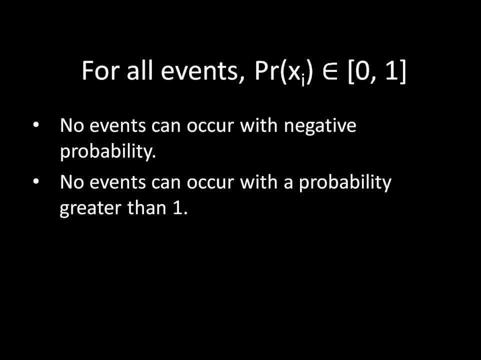 So that fails for a lot of reasons because, well, you can't have a probability occur with probability greater than one or greater than 100 percent. So if you ever had a sports coach who told you to give you 110 percent in today's game, well, you can just ignore them as being ridiculous.